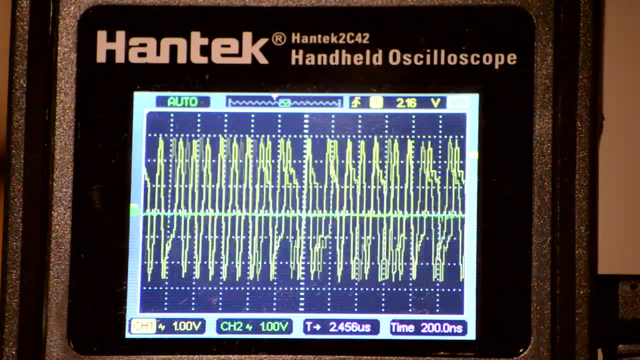 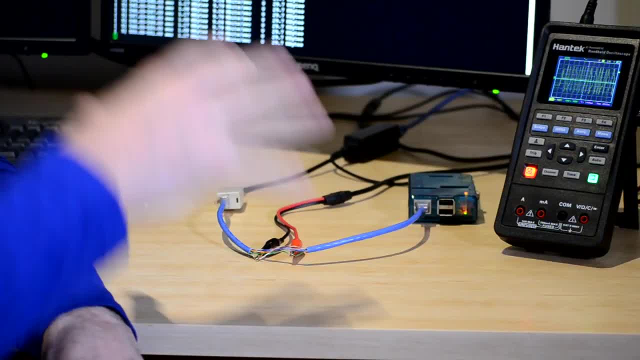 going through. now. what we can see on that scope is voltages going up and down and different widths and things, those. those are all characteristics of this 10 mega. second link: okay, I've slowed it down to 10 meg, which is pretty slow, but it makes looking at it on the scope easier. okay, but things like that too. if 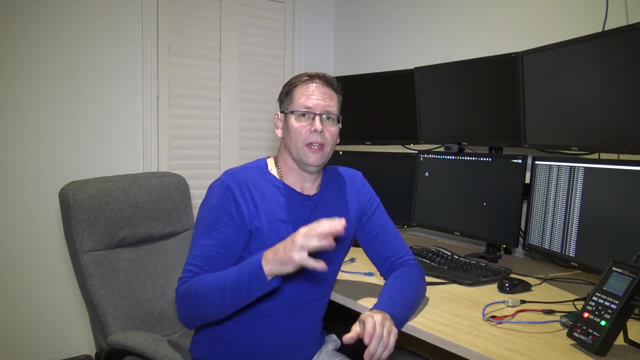 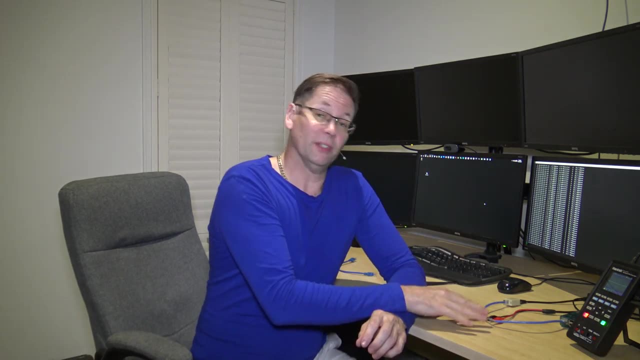 it's 10 meg, 100 meg, 1000 meg. they're all components of the physical layer, so they define what sort of coding gets, represents the bits on the wire, and at that point they're called symbols. so once it's on the wire here and you've 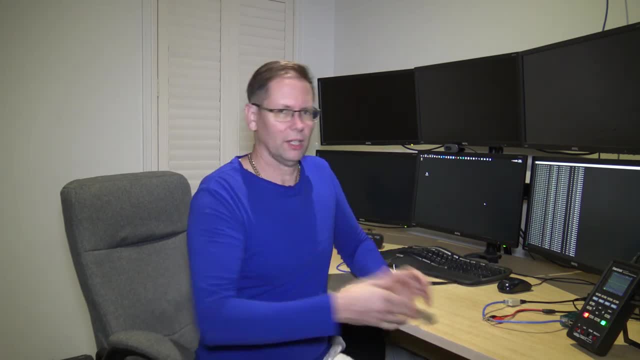 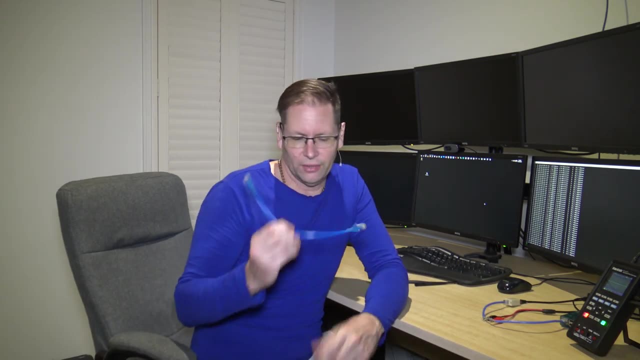 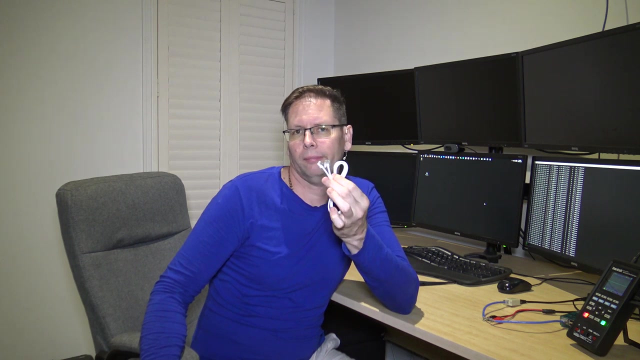 got. you might have a few bits represented by one signal change. it's called a symbol. okay, so that's just a look at the transmit coming out of the Raspberry Pi. but this Ethernet was just one example of a physical layer technology. right here got an old phone cable, nothing special, but if you remember, back in the day you had a dial-up modem. 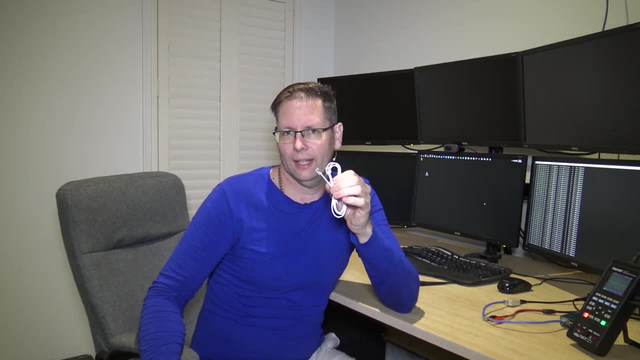 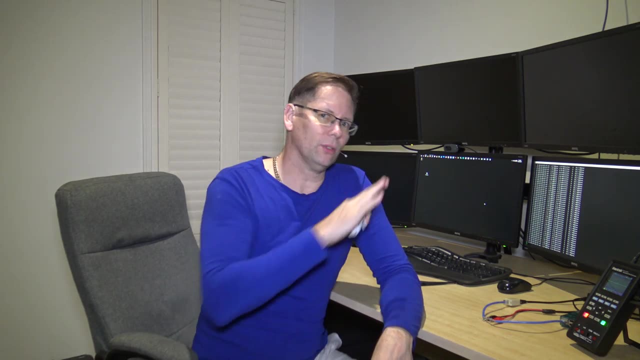 okay, you would use your modem through the phone line and connect to the internet. now, after you've done that, there's other layers above that. get you things like your ip address and you can still go to a web page, because that's all the same, but down at the lower layers it's different. so, through a 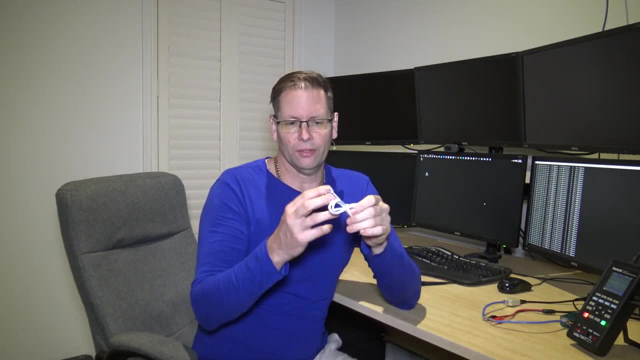 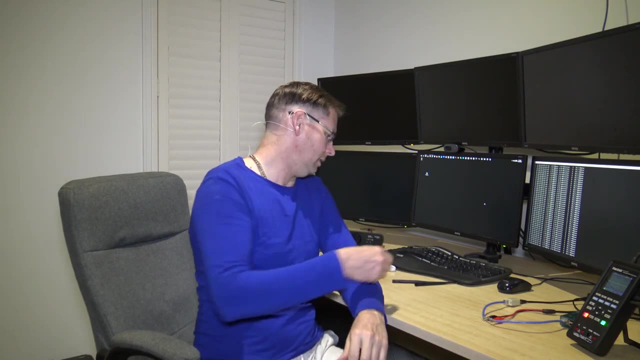 phone line. you've got different types of electrical signals. you've got different types of cable, different types of plug, different types of equipment. so that's another example of a physical layer technology. now, one that might seem tricky is when you're talking about wi-fi. okay, because 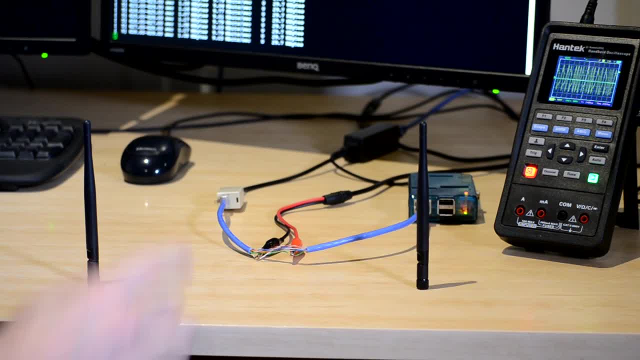 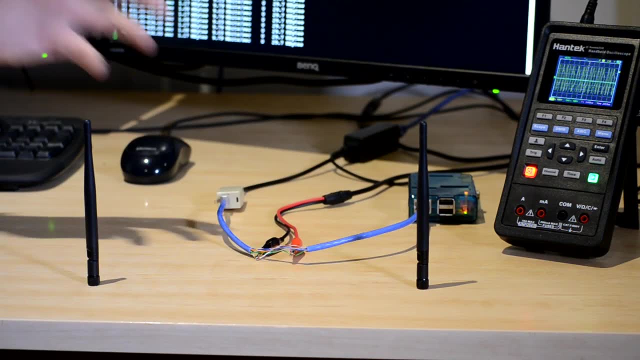 let's say you've got one host here and another one there. what's the physical layer? well, there's nothing we can touch. okay, we can't touch anything, there's nothing in between to get to physically. but the radio waves themselves are the physical layer, and wi-fi actually gets pretty interesting. 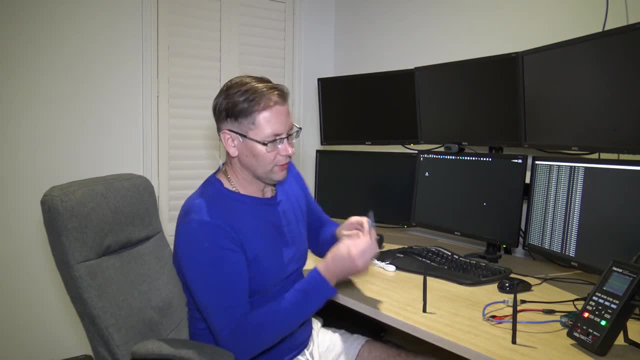 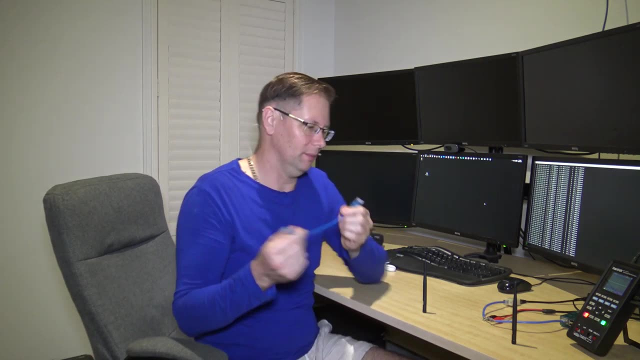 at the physical layer. so if you're talking about a physical layer, you've got a physical layer because, unlike an ethernet, where basically if you plug it in, odds are, with exceptions odds are. you're pretty right that you know you've got a good connection generally, but when it comes to